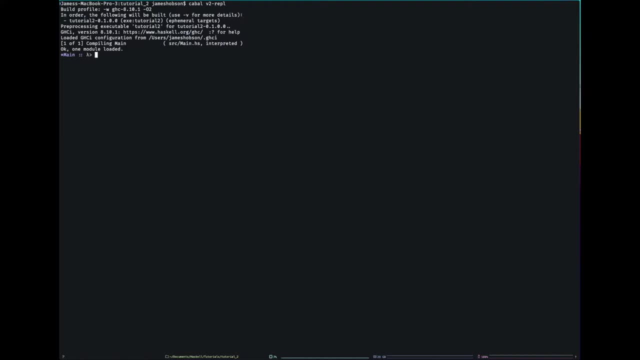 composing functions together to sort of enhance functionality. That's what you're thinking about. So, now that I've mentioned that, it's probably a good idea to talk about functions. So, looking at my screen, I just made a blank Cabal project and opened the REPL. 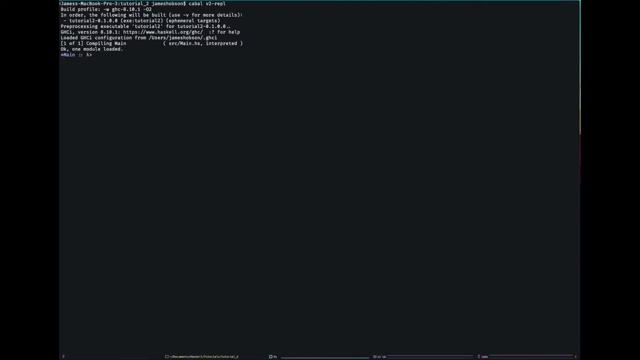 Nothing special, So right, what I'm going to do is I'm going to import two libraries: datachar and datalist. Well, I forgot the imports. Okay, so now that we have both of those imported, um, let's look at some functions. So if I type colon T, um, it's going to give me the type of whatever. 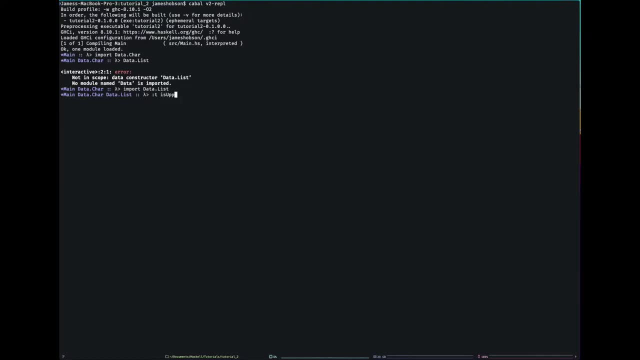 follows. So isUpper is a function in datachar that tells you it has, it gets past a character and it gets, tells you if it's uppercase or not And you can see the type is written. like that, char to bool Makes sense, Maps characters to booleans And we can test this out Um. 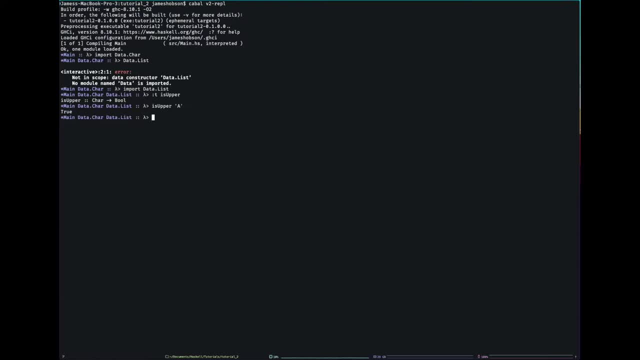 isUpper a true, ah false, Space false, one false. So you can kind of see what it's doing, Um. now notice that I didn't. I didn't put any brackets around the inputs to the function Um, and there's a reason for that. 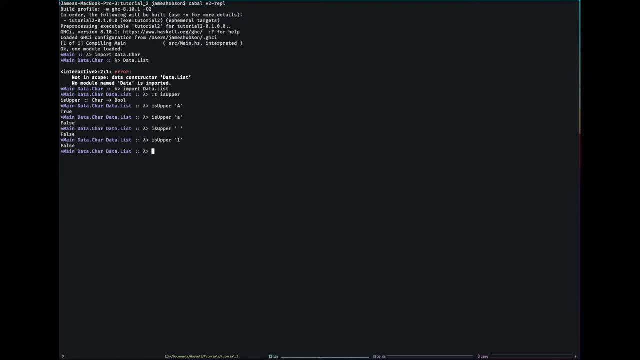 and it's because all functions take only one input. So what's the point of brackets? Now you're probably thinking: what One input? But I can define a certain number c function, for example, like this: int a, int b, you know, return a plus b, you know that's a c function. 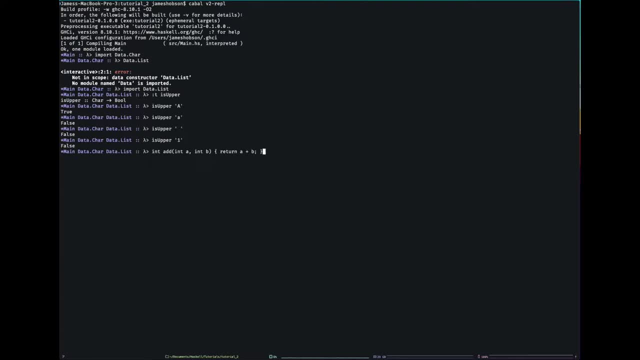 um, that has two inputs. well, the haskell is going to go. no, no, no, that's only one input. it's just, it's a tuple. there you go. it's a tuple, um, in haskell syntax it would just look like this: you know, um, now we have brackets because it's a tuple and that really they'd say that c is over. 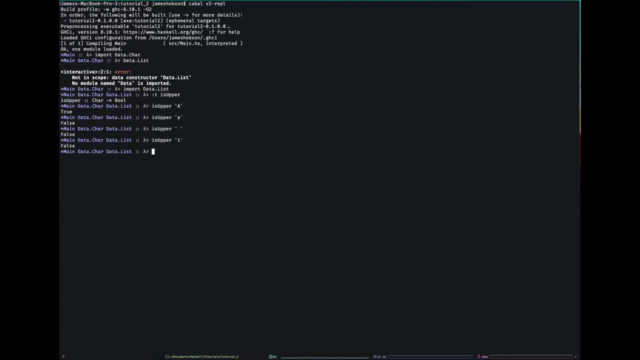 complicating it, because functions with one input, you still pass it a tuple, but it's like a one tuple, i don't know um. so i i could define a function, say uh, add int, which uh in haskell is going to take in a and b and it's going to return a plus b, and then i can go add int. 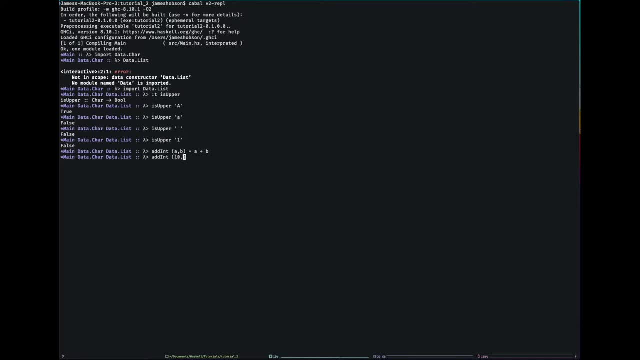 um 10 and 7, 2, 12, cool. but um, that's not really how we do things in haskell. we we've kind of abstracted. we've already abstracted um function application by saying, okay, it only takes one input. um. so what haskell types normally look like is: um. well, i'll redefine, add it. 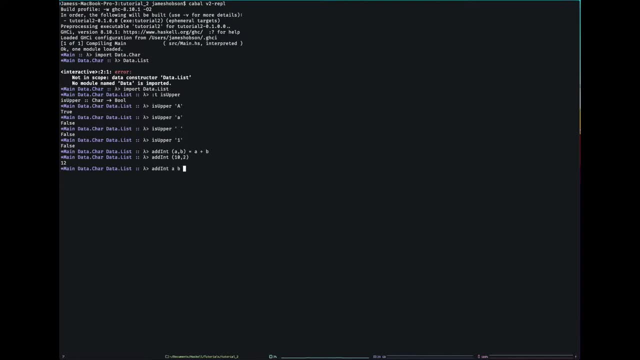 um, i'll redefine add int. so normally it would look like this: okay, um, and the type would be int to int to int. and now this seems completely unclear. what's going on? it's not clear what the inputs are and what the outputs are, but, like i said, 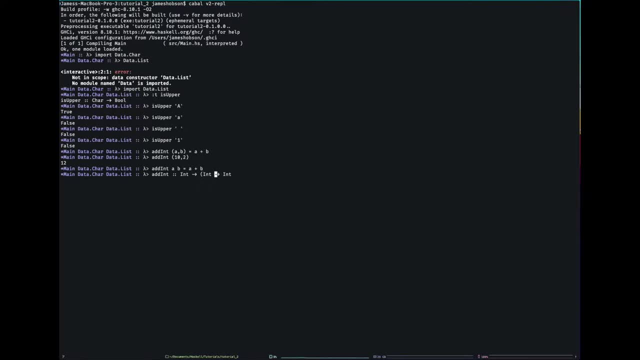 there's only one input and haskell has implicit bracketing. so what this is saying is: add int takes in an integer and returns another function which will add that integer to whatever. so we can, we can kind of experiment- that we can make an increment function which add int one. and now 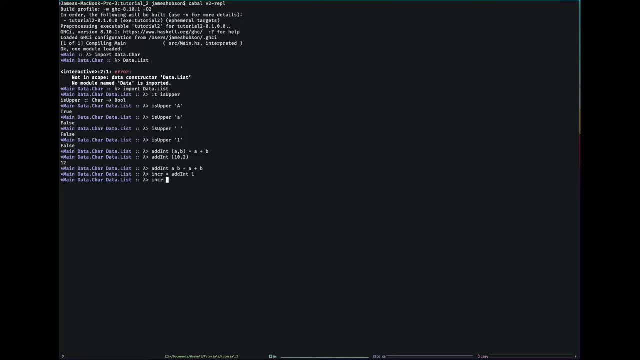 incur and then 10. it's going to give me 11 and that's called partial application. but that's add int. one returns a function that adds, that's one. cool, so great, we've, we've. we've sort of abstracted away from that, okay, um. so maybe something to mention is casing. you'll notice that all of my functions start with a. 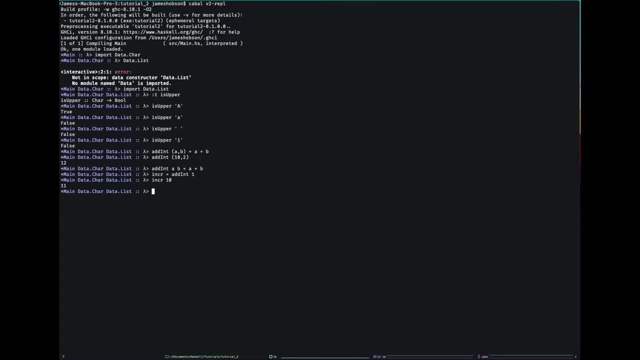 lowercase um letter. uh, they have to um, unless you're defining infix functions which are made out of symbols um. the reason for this is because types um, like int for example- you can see up here chartable- they start with uppercase letters, as do data constructors, but more on that when we cover data types, which i don't think we're going to cover in this tutorial. 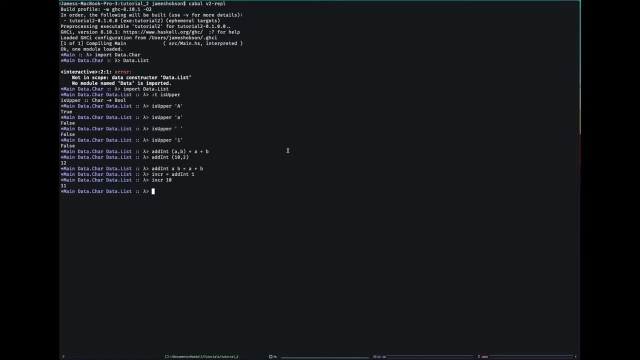 um, so great um function composition next. so i have my inker function and i want to join that. maybe i want to do it twice. what i'd do is i'd go dot inker and then, uh, this is a function in its own right. if i give it 10, it'll give me 12.. now what that dot does is it's an infix object. 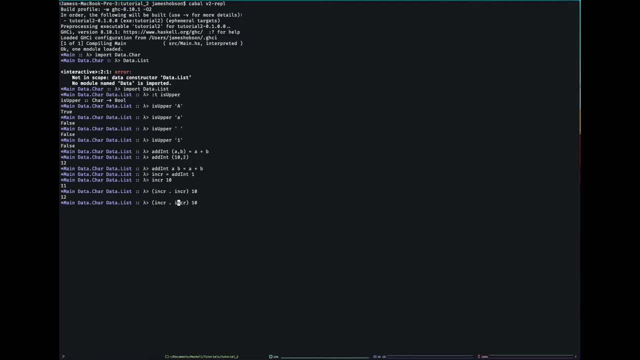 operator and it takes in two functions, this one and this one, and it and it returns another function that passes the input to this one and then the output of that one gets passed into this one. um, and this is kind of how you build programs in haskell. you use function composition, um. you. 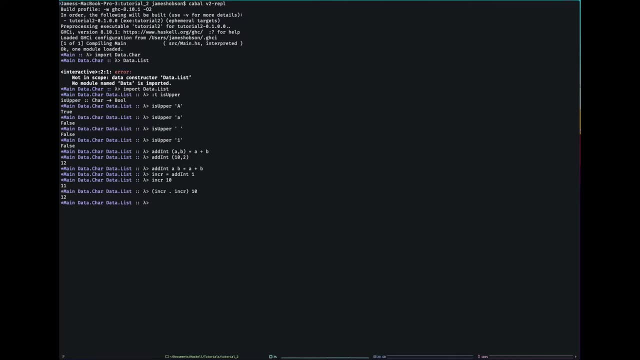 compose functions together to sort of extend function, add functionality to your program. um, great. so next thing maybe to cover are lists. so lists on are linked. actually, in haskell by default, um, there are libraries that will give you arrays and vectors, but, um, it makes. it makes a lot more sense. 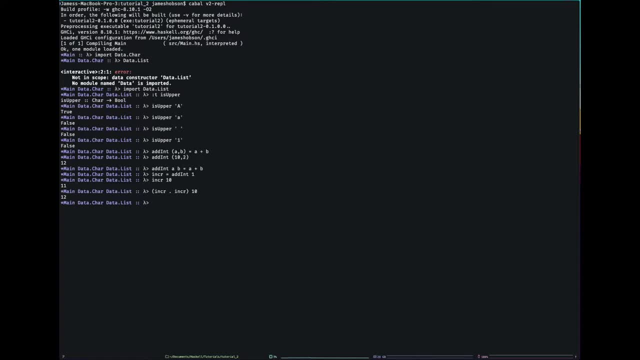 in haskell to think about linked lists, and the reason for that is because haskell programs don't have state. they have, um, no, no such thing as a variable, and so going through arrays is quite difficult. um, because you, you can't really keep track of where you are in an array. everything's done through. 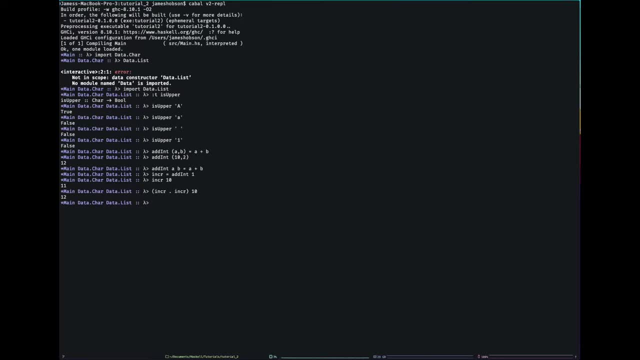 recursion. um. so it makes a lot more sense to think about lists as linked, but i define them a bit like an array. here's a list one, two, three. um, i can join lists together with plus, plus. oh well, i'll do. um, i can add to the front with: 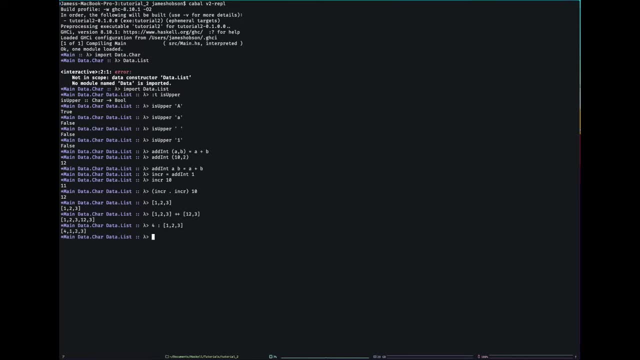 colon um that's gonna write the join operator in the linked list. we're saying four is attached to that list, um, we call it cons, um, but it's colon um. there's also list comprehensions, um, and ranges. so ranges are quite cool. if i go one dot dot ten, you can get the list one to ten, um i could go. 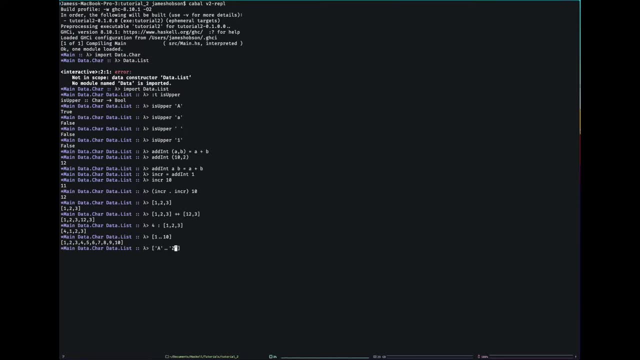 character a dot dot, character z. and now i'm gonna get you know that string which is just a list of car uh characters. um, what else? um, i can have infinite lists in haskell, so if i don't add an end, it's just gonna keep on going um, and the reason you can have, you can, you can use them in code. 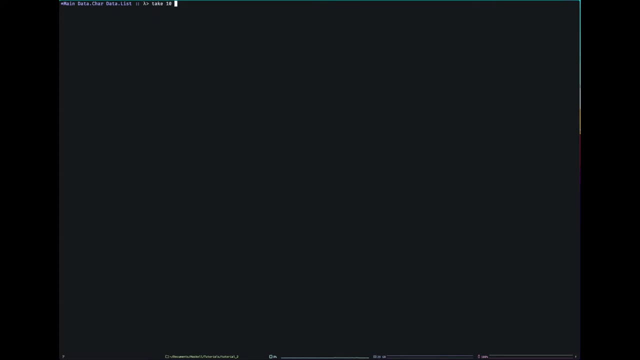 um. for example, take 10 returns, the first 10 elements of a list, and you can see it accepted: an infinite list. just fine, um. the reason for that is because haskell is a lazy language, so it doesn't compute anything until it has to um, and then, once it has computed, 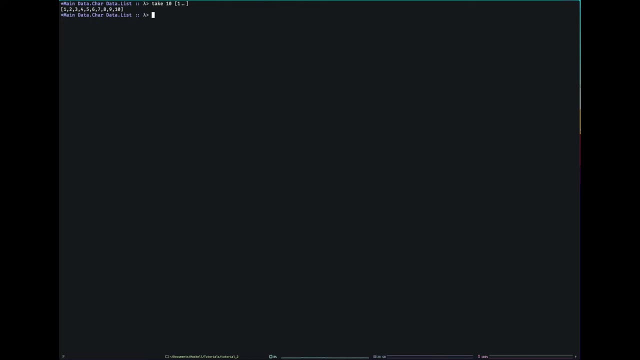 it tends to remember it. so, um, that's why you can have an infinite list. if i go x, x's equals that. um, that was just fine, because it didn't evaluate the infinite list. it decided it didn't need to um. but if i force it to evaluate x's, then it has to evaluate that infinite list. 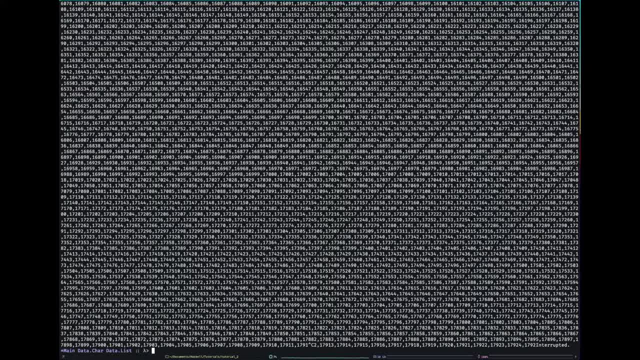 um, and it has at this point remembered that x's the what x's is up to what's that? 1792, um. so, and the reason for that is, uh, the reason it was forced to evaluate, it is because when i, when i wrote just x's, the repl went: okay, we need to print. 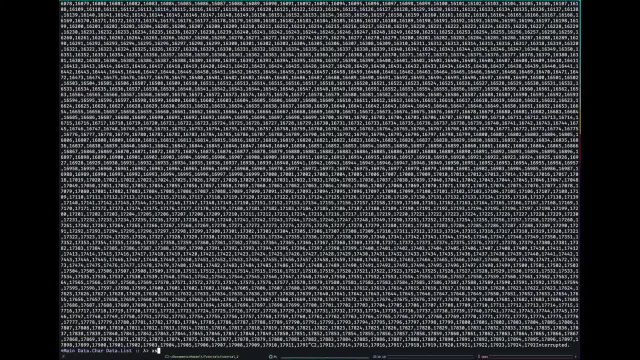 this list. what's the first element? oh, i don't know. let's work it out. oh, it's a one- great, we've printed that. now what's the next one? and it sort of evaluates in that order. now you can do um quite powerful things with list comprehensions in haskell, so, um, let's clear that again a bit of. 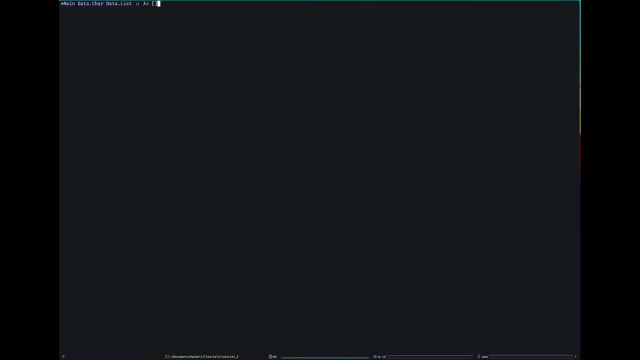 a nightmare to look at. um, so let's define a function map. there is a map already. it works exactly as you'd expect. map plus one, one to ten, adds one to them all. but we're going to redefine this using list comprehensions. so map, i've got to add the prime because i can't redefine standard functions. 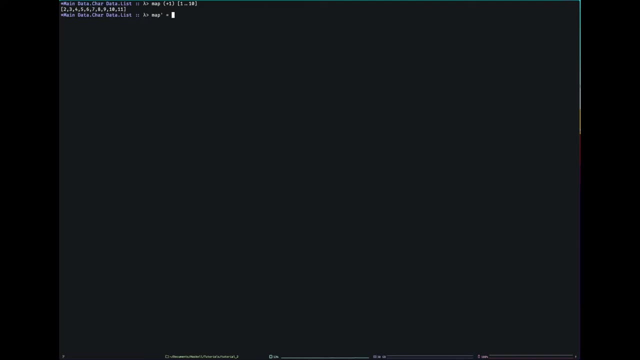 in haskell. so what it's going to do is it's going to take a function, it's going to take a list and then we're going to use a list. comprehension. so i'm going to say: it is that function with n as an input, where n is simply x's. you know, one at a time, and that uh. 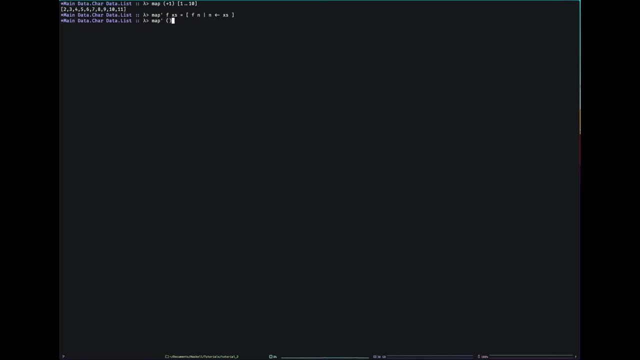 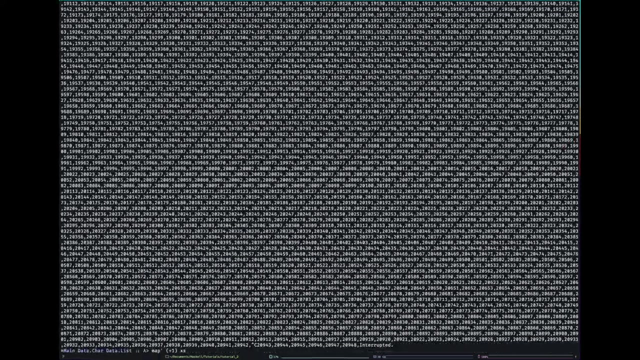 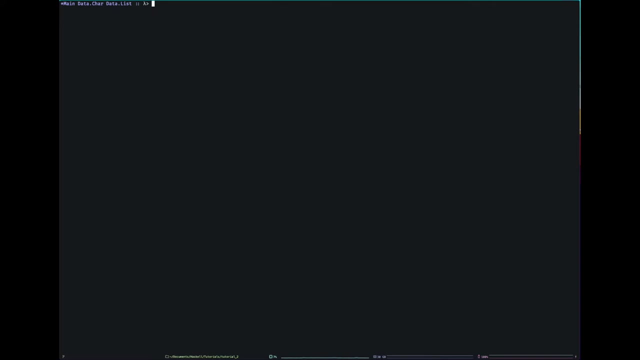 that gives me map prime, map prime plus one x's cool, oh, i forgot. x is the. uh, the infinite list. uh, one to ten. okay, there we go. um, that's, that's nice, so that's. uh. yeah, we're going to go with that. we can also add sort of um predicates, so filter, for example. let's redefine filter. 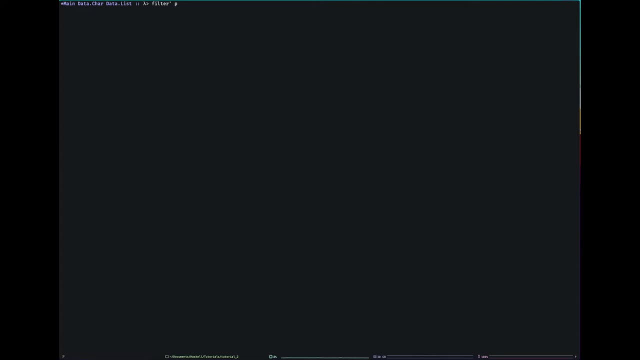 filter takes in a function that maps a value to a boolean, it's like a check? um, and it also takes a list, and what we're going to say is: it's just n where n is going to be coming out of x's and p? um p? n has to be true. so now, 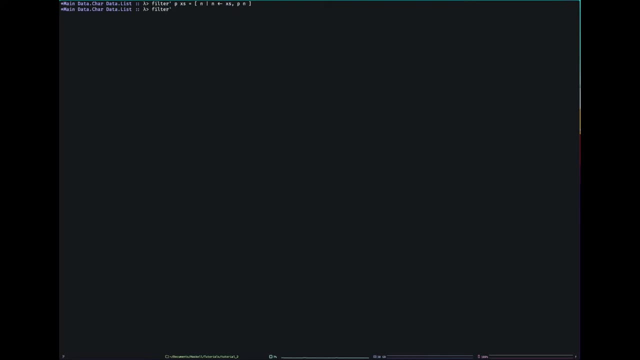 let's say we're going to say filter is even, i think it, or is it just even? yeah, it's even. so that's a function that takes in um a number and returns true, if it's even. and we're going to give it one to ten again, lovely um. 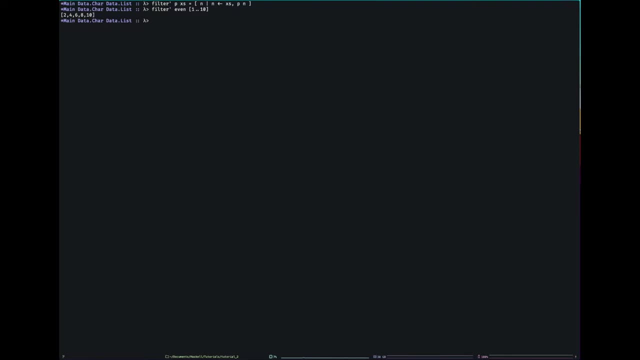 cool, so that's. you'll notice that list comprehension is. the syntax is a lot like um, the concept comprehension in mathematics. haskell borrows a lot of its syntax from mathematics, and for good reason. you know, the syntax of mathematics has evolved over hundreds of years. 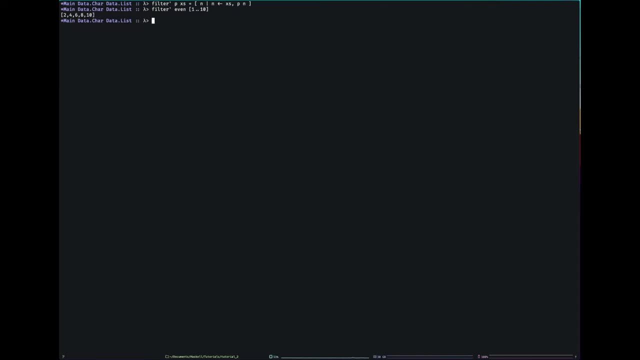 maybe more um, and so it's very ergonomic and so it makes sense to sort of steal your syntax from mathematics. it's going to be nice, um, cool. next, i think, uh, the next thing is probably: let's make a sample program, so let's make one. ah, okay, let's make a program that counts um character frequency in a string. maybe you? 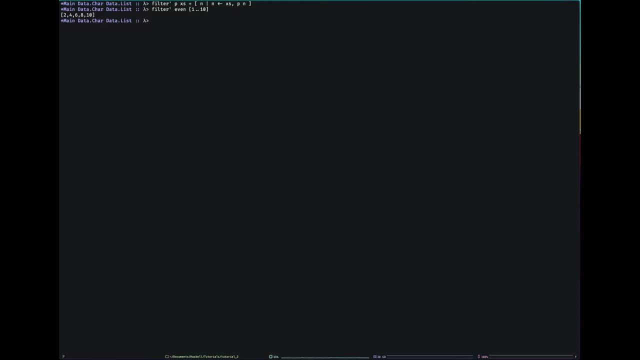 want to analyze a language. i don't know. i don't know why you want to do this, but uh, it's quite cool because we've not learned much haskell, but we're going to make quite a useful piece of code out of it. so colon e, um, that's going to let us edit our haskell function. so 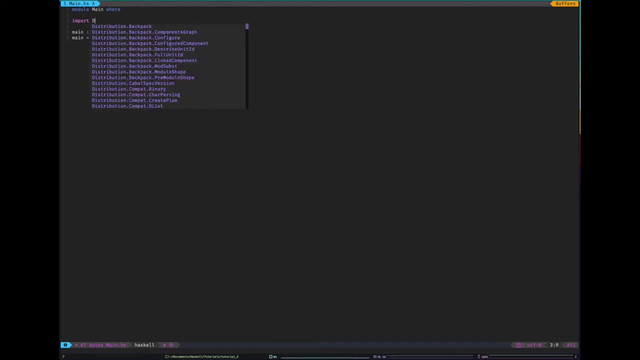 i'm going to have to start with those imports again: datachar, import, datalist- um, i didn't really show you anything from datalist. i thought i would, but i didn't. but i'm going to use it now. so we're going to define a function. 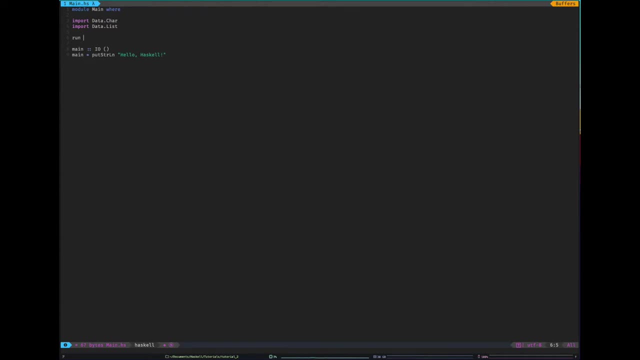 run and that's going to sort of. it's a bit like what main will be um when we get to what all this i o stuff means um, but run. we're just going to call from the repl and its type is quite easy. it's going to be string two and then how i think we should output this is a list of tuples um. 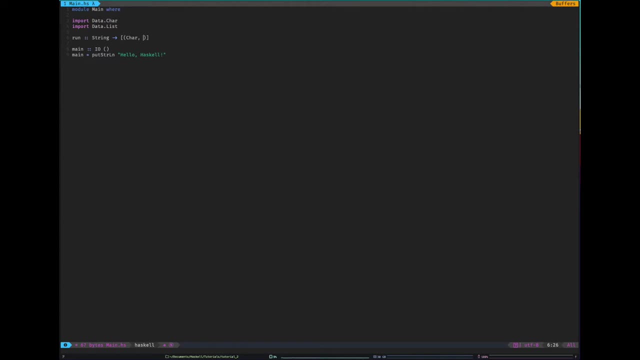 where we're gonna have a character and how many of them there were. okay, okay, now, okay. so the first thing i think we need to do is we we should probably count uppercase and lowercase letters as the same thing. um, so what we're going to do is we're going to have this function called. 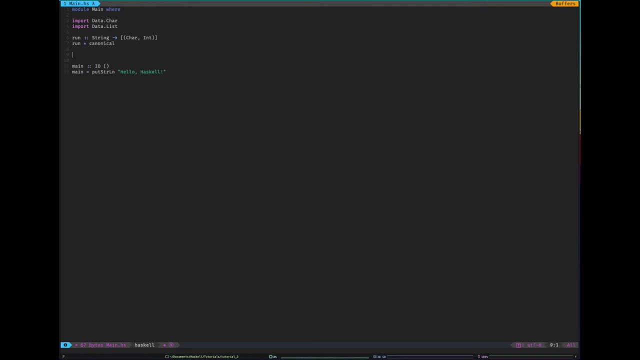 without a p. i don't know if that's how you spell canonical, um canonical, let's define it now. it doesn't matter if i define functions, uh, above or below where they're called. it's um hoisted, i think the term is. so what that's going to do is it's going to map string to a string. 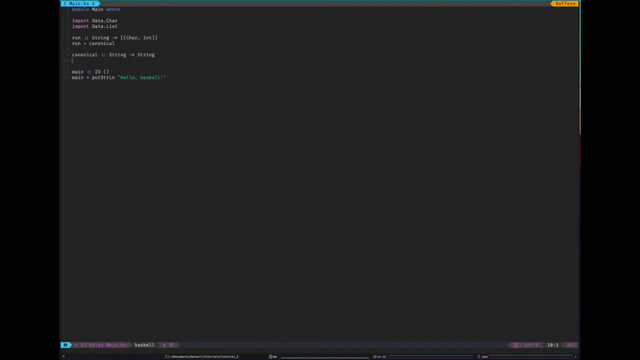 and what that's going to do is say we are given um a lowercase letter, it'll leave it alone. say we give it an uppercase letter, it will um make it lowercase, and if we're given anything else, we shall ignore it. so so how i'm going to do this is i'm going to say i'm going to start with a filter. okay, 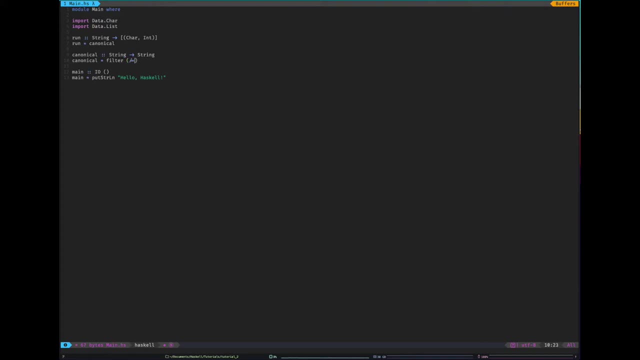 and what i'm. what i'm going to do is i'm going to filter out all the spaces. um. yes, so that's how you do not equals, it's not exclamation. equal. oh, i've got a funny font. it's not like that, it's um slash, okay, so i'm filtering out everything that isn't. 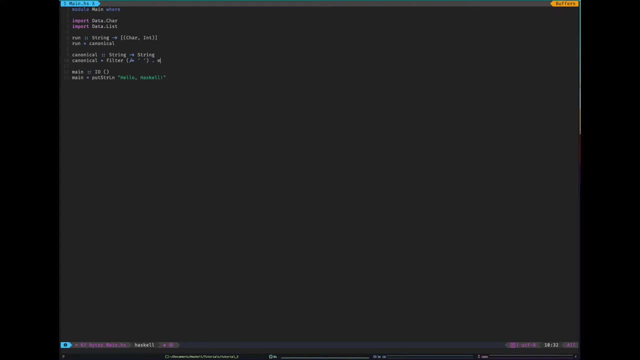 a space. and then what i'm going to do is i'm going to map over normalize. so i've not defined normalize yet, um, normalize. what this is going to do is this is going to map a character to a character. it's going to put every character into its canonical form. 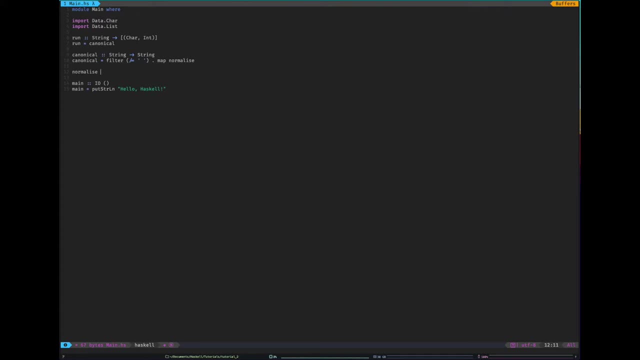 now i'm not going to bother defining the type. i don't need to. haskell has type inference. you only. you use type definitions if you want to document your code, if you feel it's necessary, or if haskell breaks and asks you to, or if you're doing a lot of type level programming, which is 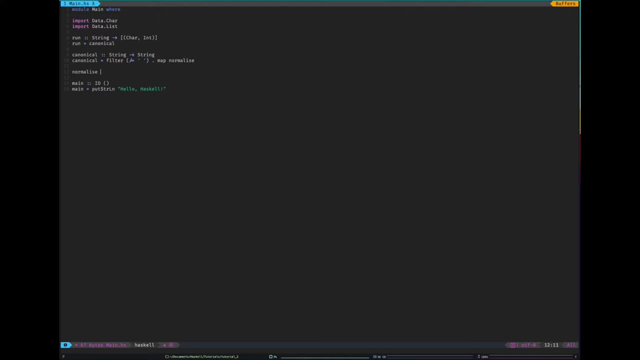 a long way, long way away in this tutorial series. but anyway, normalize. so i'm going to show you something called guards. it's a way of doing conditions, so it's going to take in a character. um notice here, though with canonical i didn't actually um specify it had any inputs. 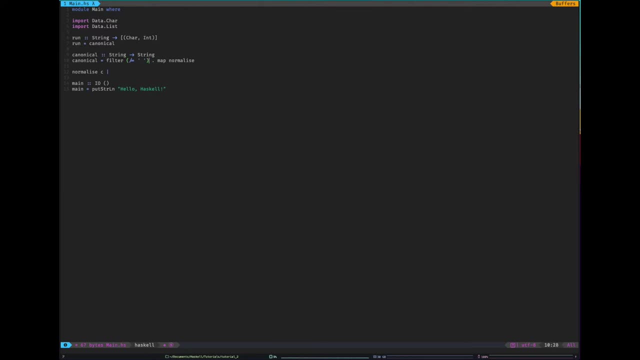 um, and that's because i'm using function composition. so remember, filter takes in a predicate and a list. a map takes in a function and a list and returns a list. they both return lists. so what this is. what's happening here is i'm taking map and i'm giving it a function. so now the type of i'm going to 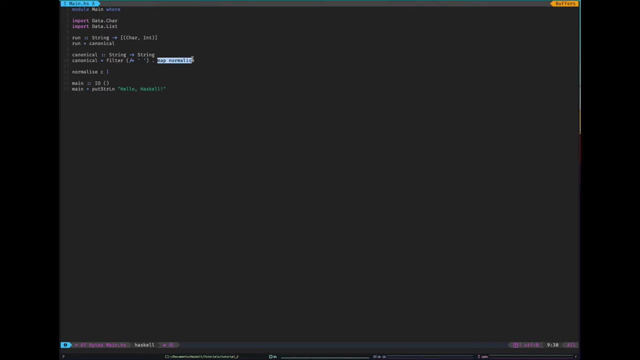 use my mouse. the type of this is list to list filter takes in a predicate and a list. we've given it a predicate, so the type of this is lists- list, and then i can compose them together with dots. there's no need to give it an input. with normalize, i am going to 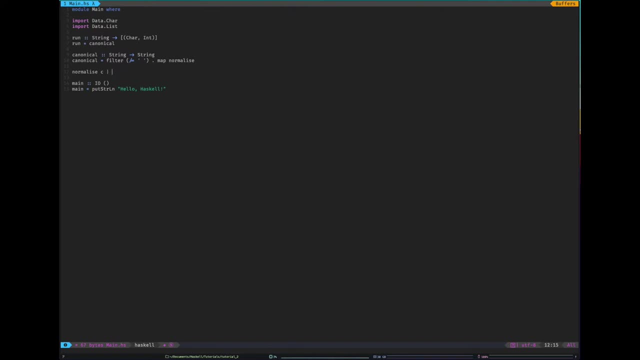 have to give it an input, so c. so what i'm going to do is i'm going to use some of those functions in datachi. i'm going to say is upper and this line here, this pipe is a guard, so what comes after is a condition, a boolean condition, and it's going to run that line, if it's true. so is it? 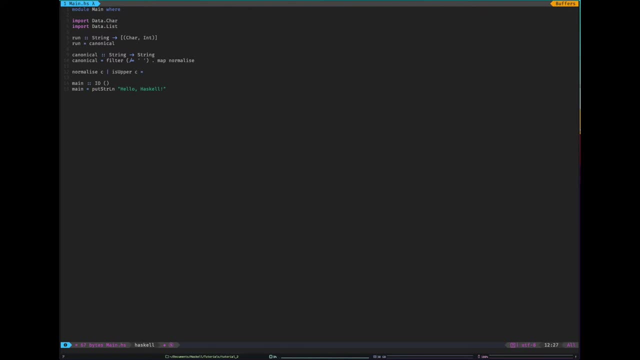 uppercase. um, i'm going to say we'll keep all the ones uppercase, so we'll just return c. uh, no, whoops, i don't need to write that again. okay, so the next condition is: lower c equals. and now we're going to go to lower c. so, uh, to lower just makes an uppercase thing. 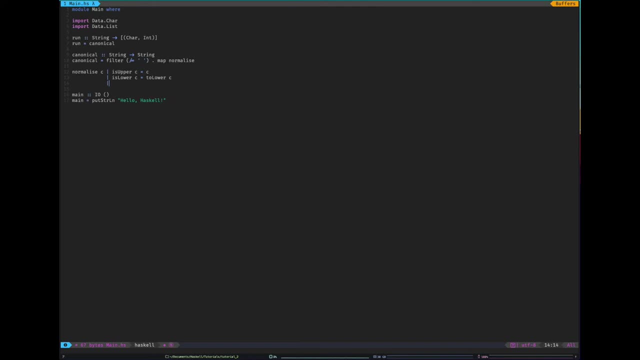 lowercase and then finally anything else. oh you, that aligns so nicely, so otherwise it's sort of a catch-all case. um, we're just going to output space and that's because space is filtered out. um, cool, so i have this function canonical. let's see if i made any mistakes. 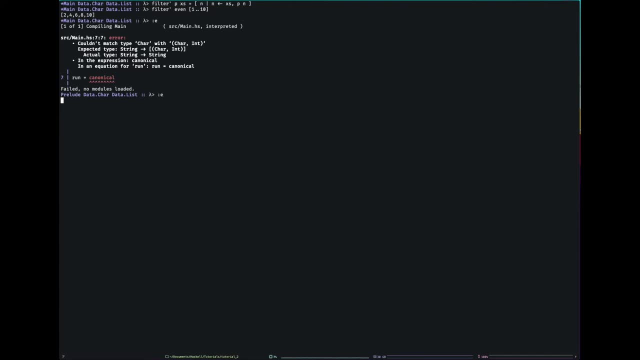 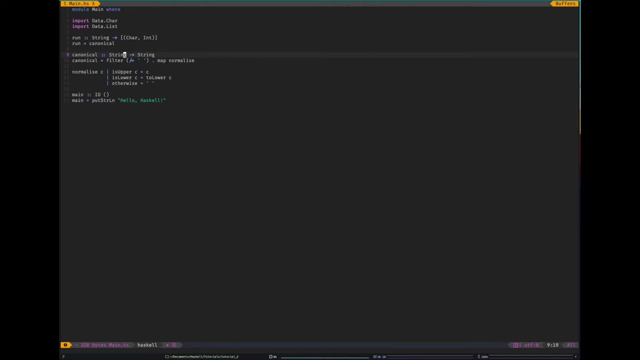 um, oh, interesting, canonical, oh, string to string. what did i forget? normalize? what's it saying? couldn't match type child charts? oh, of course it's because, uh, canonical is string to string and i've said: this function is string two, and then something else. um, what i'll do for now is, um, i'll say undefined and comment that out. so that's, that's quite um. 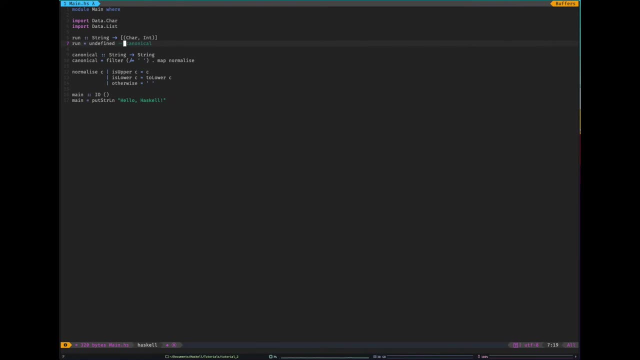 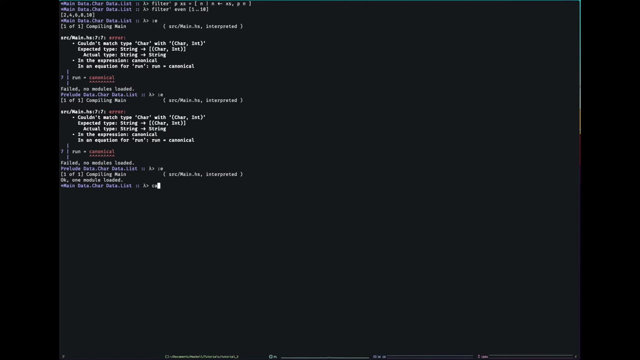 quite a nice feature of haskell is that it is so strongly typed that the joke is: if it compiles, it works as intended. you don't really get runtime errors. now it won't complain and it hasn't good. so, uh, let's try this so canonical and then let's give it a string. hello world. so we've got some. 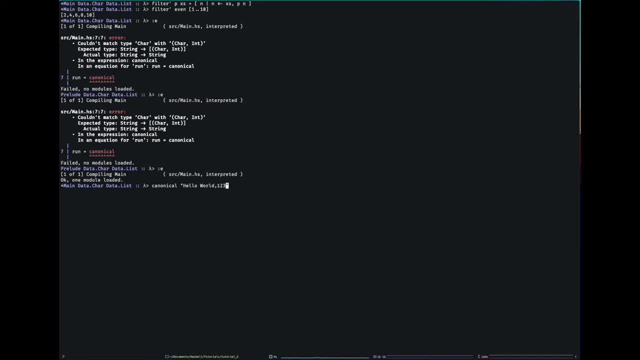 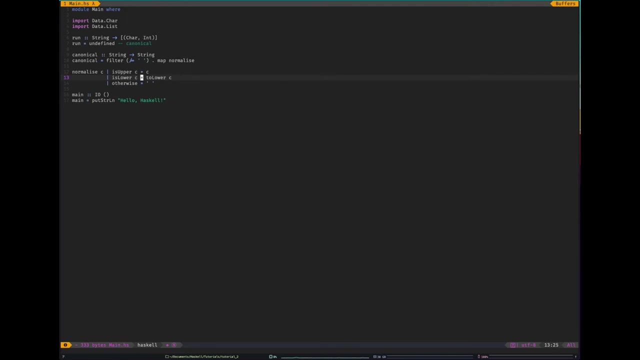 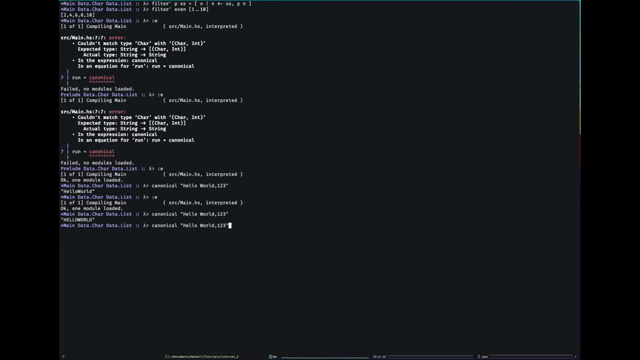 some and i'll give it some punctuation, and now we just have hello world. oh, interestingly, it's kept the uppercase. i don't want to do that. um, um, ah, whoops, um, to upper, there we go, much better, okay. so now that we see, so i'm showing you how to debug. 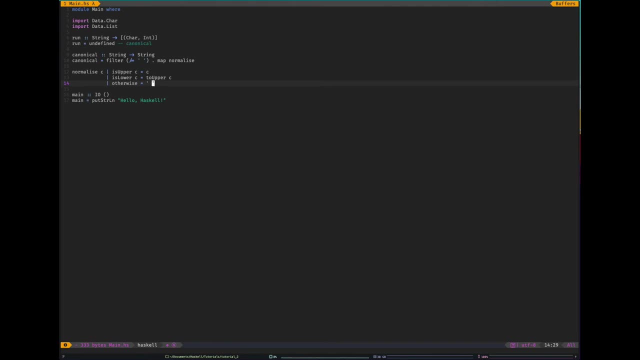 um code as you go along using ghci as a repl. it's very useful, okay, so the next, the next step would probably be to sort the letters um. so what i'm going to do up here is i'm going to say um sort dot, canonical, um so chart. 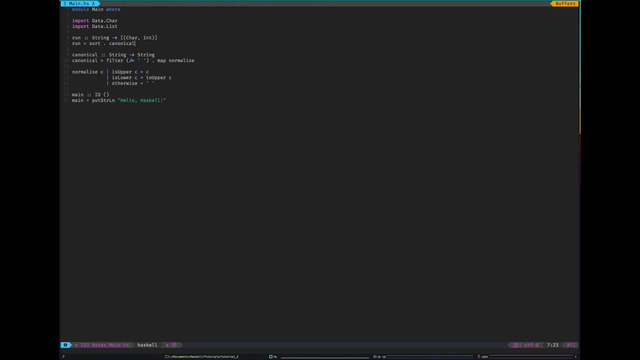 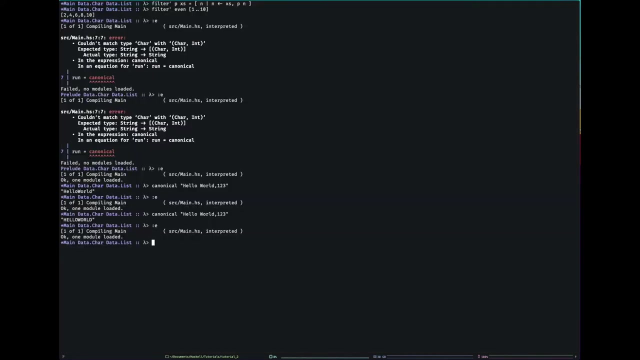 they can be ordered. you know, a is less than z and it means that we can sort that list, and sort is provided by datalist um. but i'm going to undefine this again because i want to show you another function called group. so group is an interesting function. 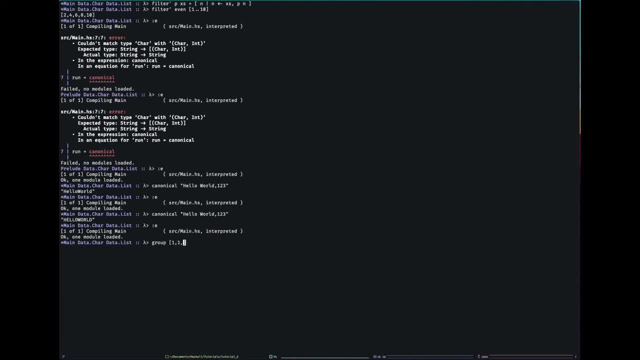 um, let me show you what it does. if i give it maybe a list 1, 1, 2, it's going to group that into 1: 1. so it's a list of lists 1, 1, 2.. if i give it another 1 here, you see that's in a list of its own. 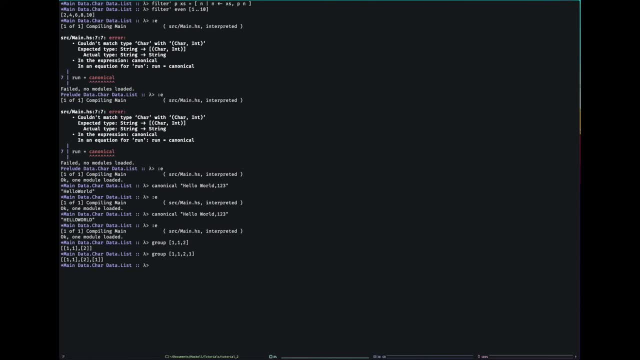 and that's why i've sorted the list um. So the idea is that essentially, if I go groupsortcanonical and if I say f equals, and if I go f hello, then yeah, it's quite nice. That's how we're going to do the letter frequency basically. 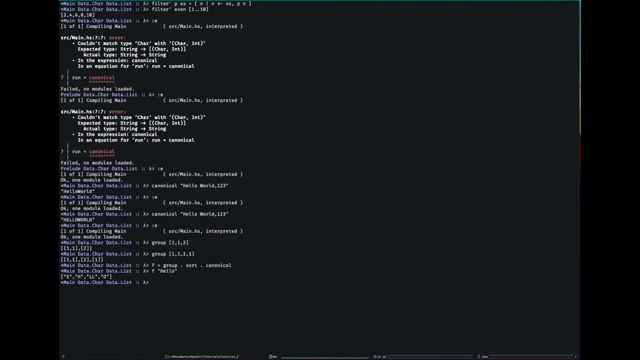 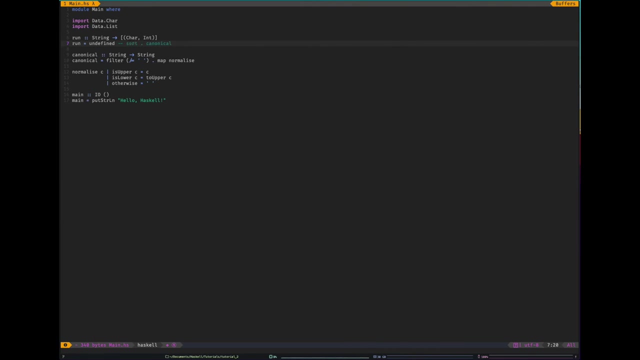 So the final step would be to count how many things are in each inner list. and count how many things are in each inner list and char int. Okay, so display it well is the answer. So what I'm going to do is we've got sort and then group. 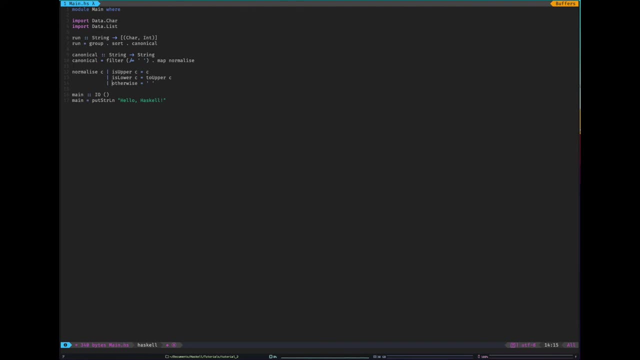 And then I'm going to make something called display. Now what we're going to do is we're going to map over our sorted and grouped list and we're going to use a lambda here. So lambda's in Haskell Backslash is how we backslash in the input.